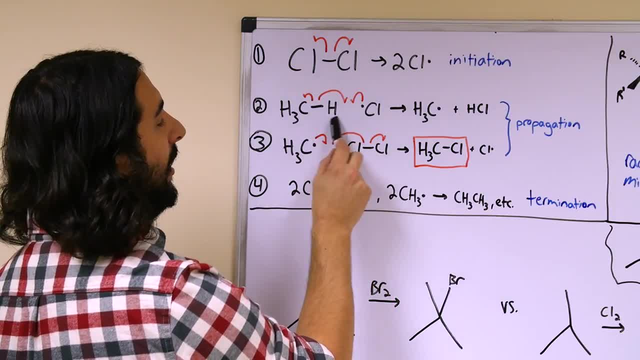 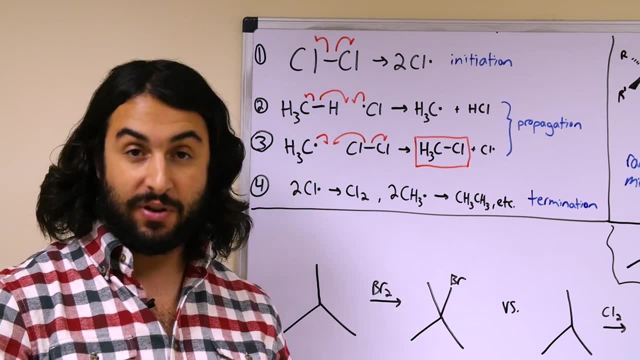 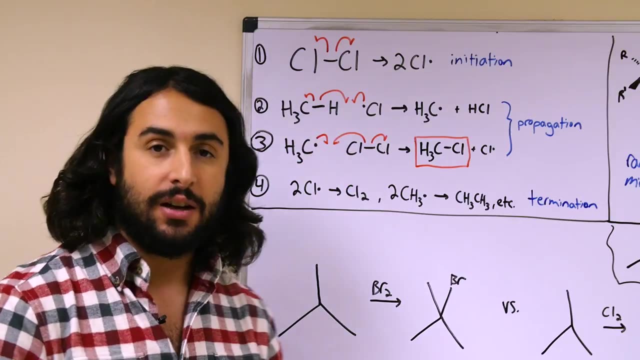 these electrons will go here and a hydrogen radical will now make covalent bond with chlorine, giving us HCl and leaving us with, in this case, a methyl radical, which can be very unstable. and so that means that, now that we have a methyl radical swimming around, if it finds another molecule of chlorine, it is going. 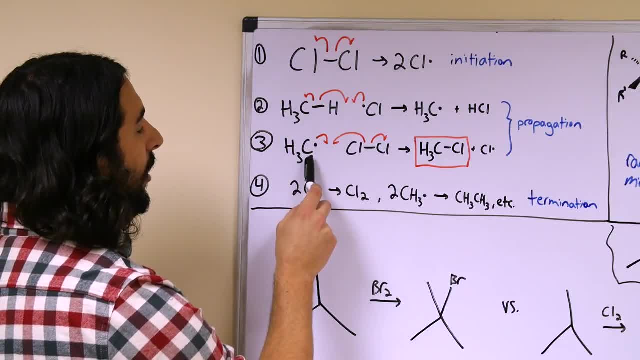 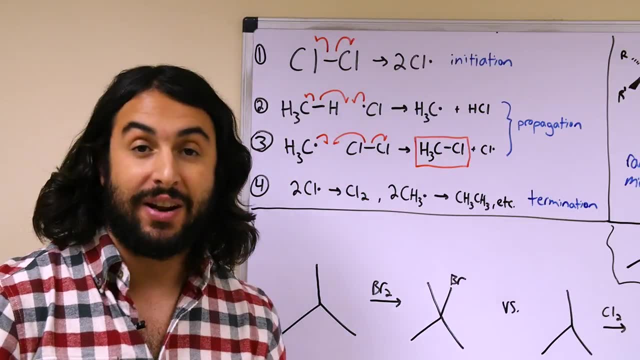 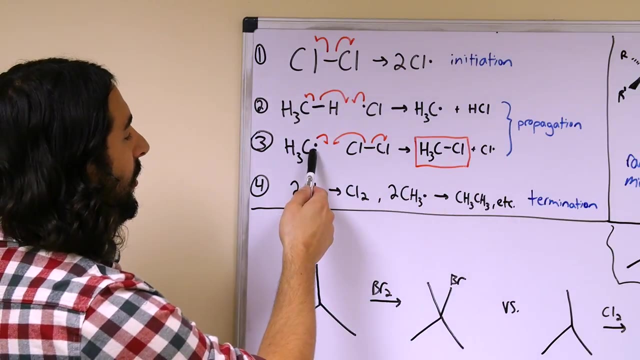 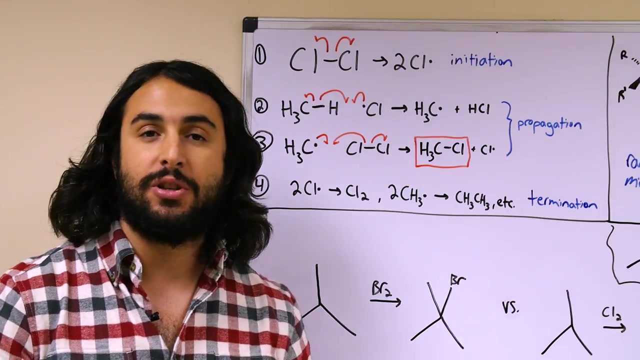 to propagate further and go ahead and reform a carbon-chlorine bond, leaving a new chlorine radical, and so this is our chlorinated product and in this case, was generated in a propagation step. it is just as well that a carbon radical could have found a chlorine radical and then the chloromethane could have been. 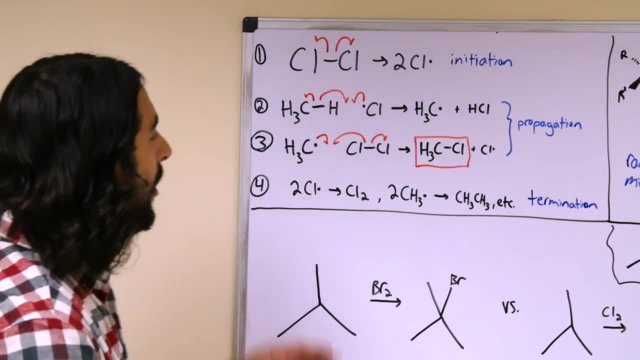 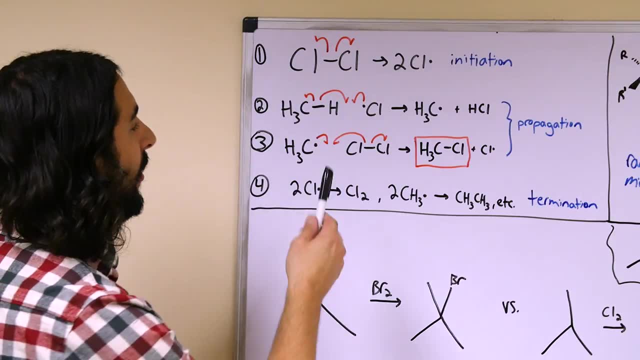 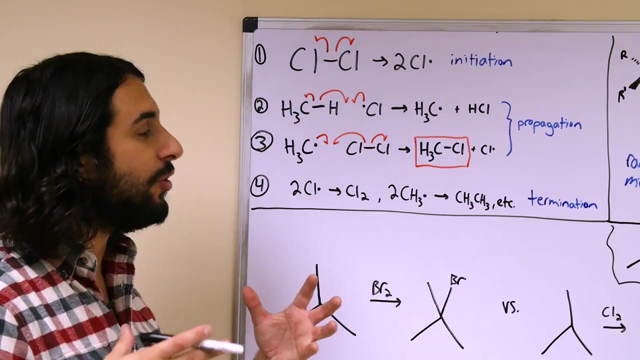 generated in the termination steps. so there's a lot of ways for this to go, but in this case we do it as a propagation step. and then any two radical species that you could find in this system, whether it was two chlorine radicals, two methyl radicals, a chlorine and a methyl radicals we just said. if any of those, 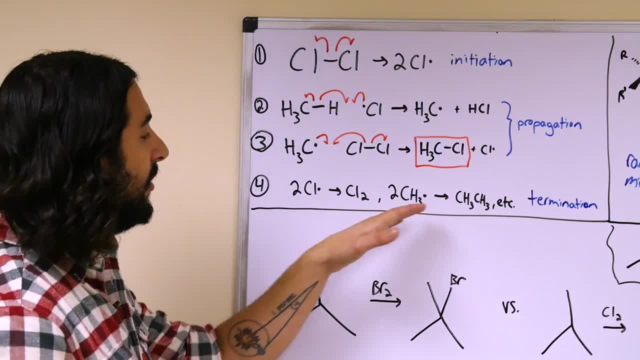 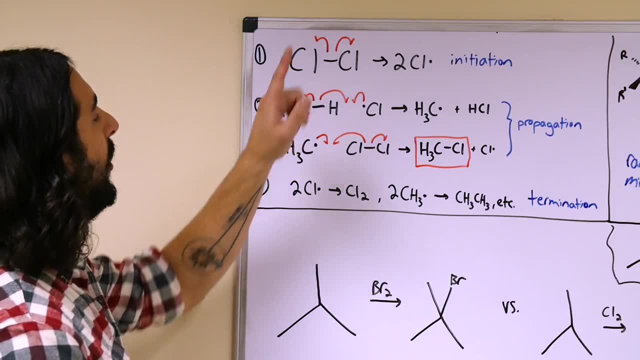 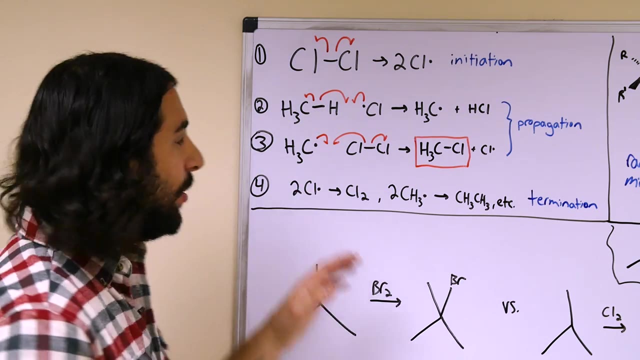 were to collide, then they would form a covalent structure in a termination step. so this, let's just remind ourselves: we're forming chlorine radicals. the chlorine radical is going to propagate some alkyl radical and then the alkyl radical will want to bind to anything you can find. so if it runs into a chlorine molecule, 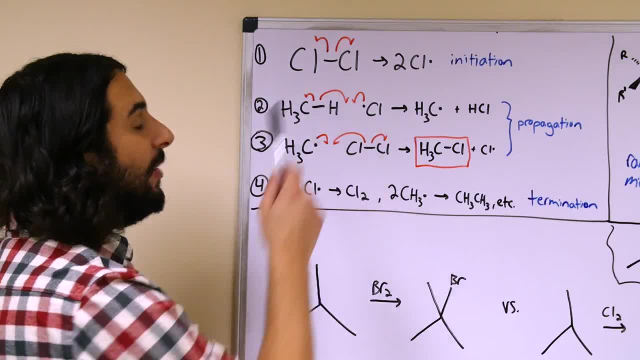 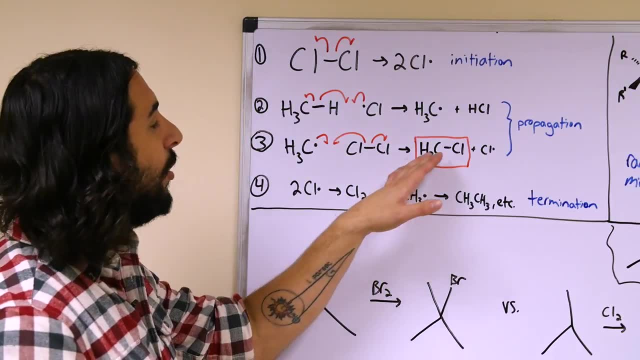 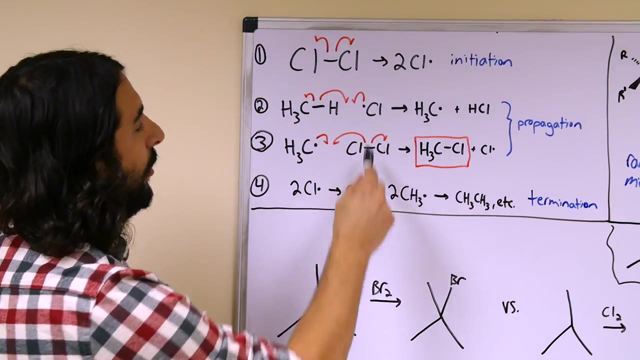 which is probably much more prevalent in the system than chlorine radicals- being very unstable, then it will go ahead and form the monochlorinated product. now, the monochlorinated product can then go ahead and react further. if this structure comes into contact with another chlorine radical, that chlorine 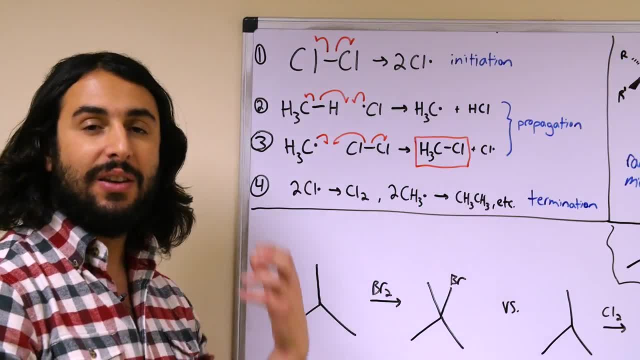 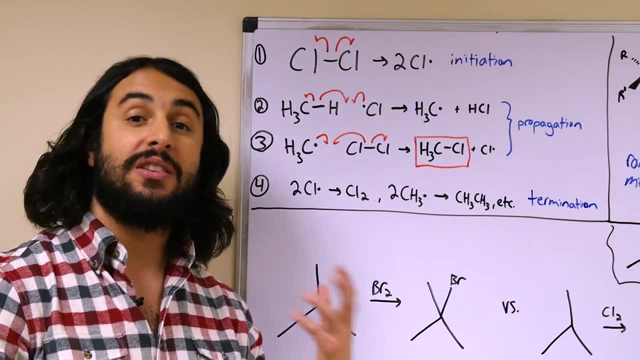 radical can strip away another one of those three protons, leaving another radical that can get another chlorine. so then we could have a dichlorinated or a trichlorinated or even tetrachlorinated, so we could have tetrachloromethane. 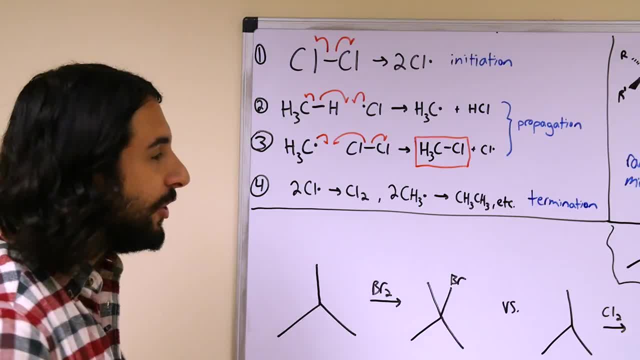 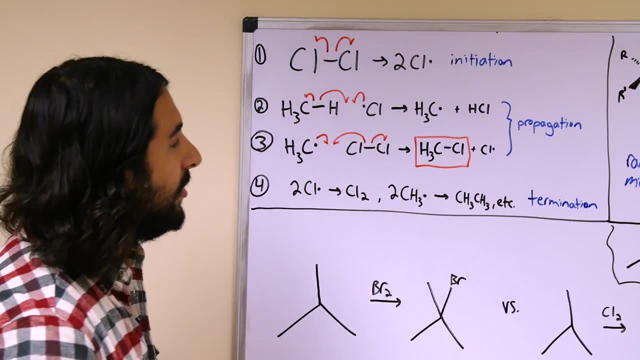 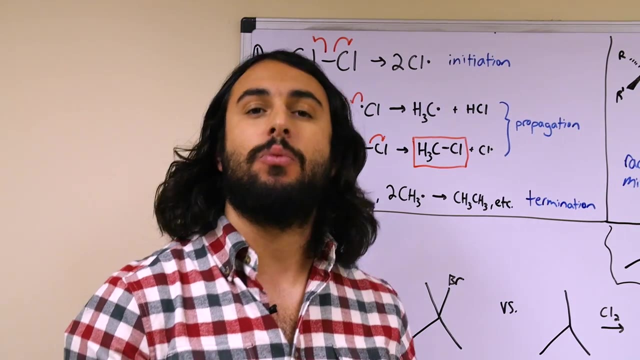 and so that's how halogenation works. for for alkanes it's going to have to be a radical mechanism with initiation, propagation and termination, as we see you now. another thing that we got to understand about these radical mechanisms: remember when we were looking at, let's say, an SN1 reaction, where we 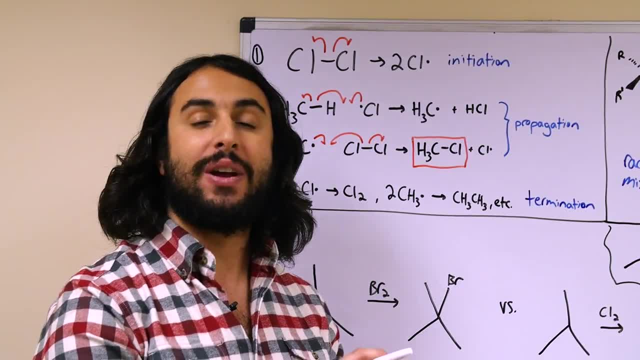 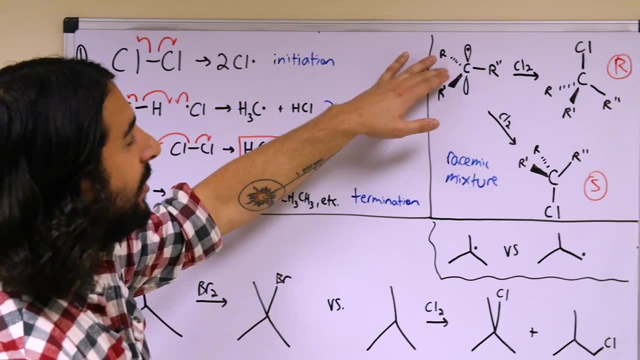 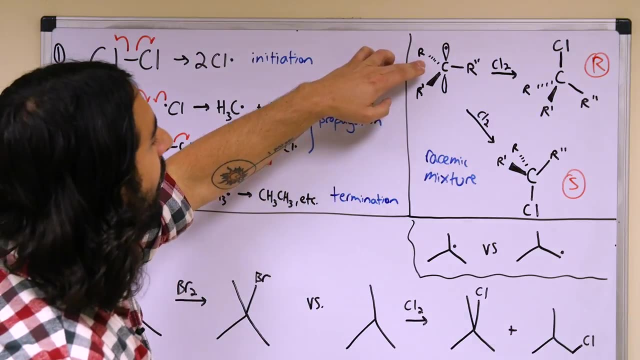 had the sp2 hybridized trigonal planar carbocation intermediate, we had to be aware of the possibility for a racemic mixture because when you have a planar situation like this and recalling that a carbon radical is also planar and sp2 hybridized, that means that let's say we have this carbon radical and let's say 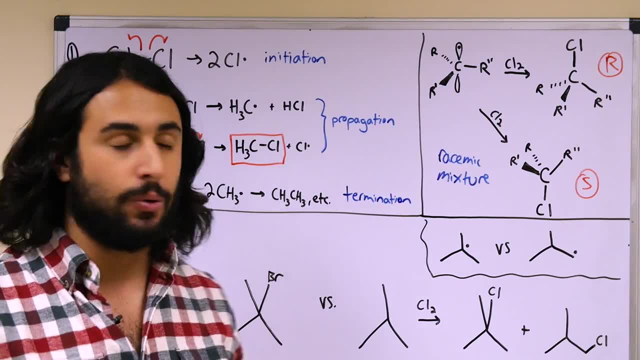 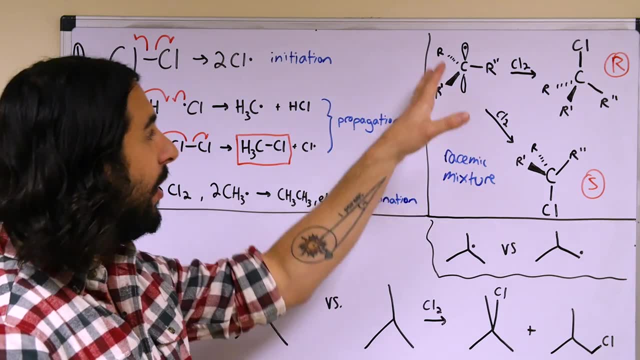 we have three different groups here. let's say they're just three different alkyl groups. so that means we have the potential to form a stereocenter. if that carbon binds to, you know, forms a bond to a new group. and so let's say we have a chlorine molecule. let's say the chlorine molecule is going. 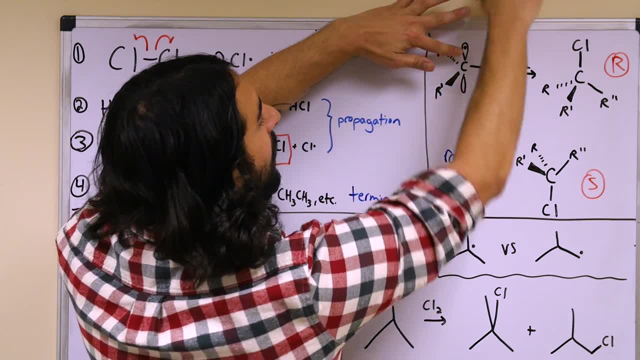 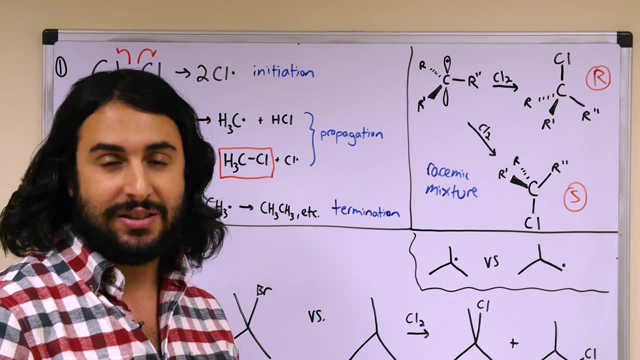 to approach from the top, and then we're going to generate a carbon-chlorine bond. the other chlorine radical will go away, so we have a new carbon-chlorine bond. so there, that is here. but then let's say similarly, it could approach from the. 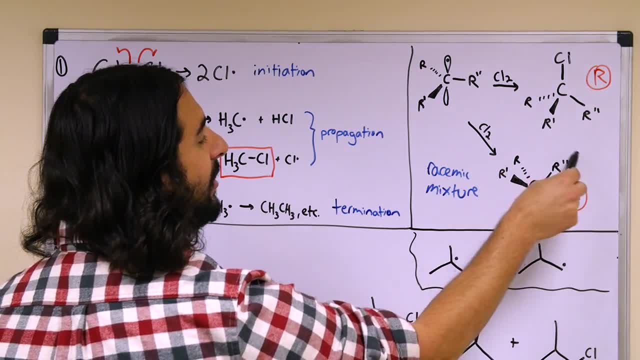 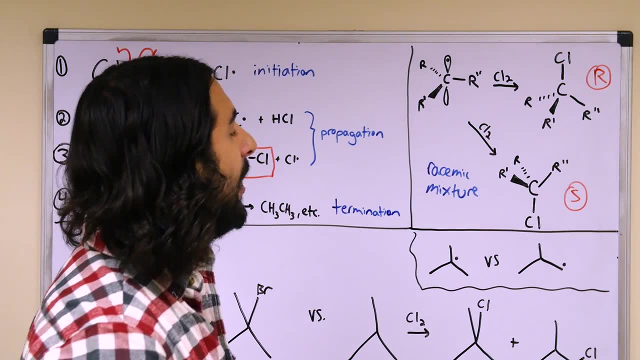 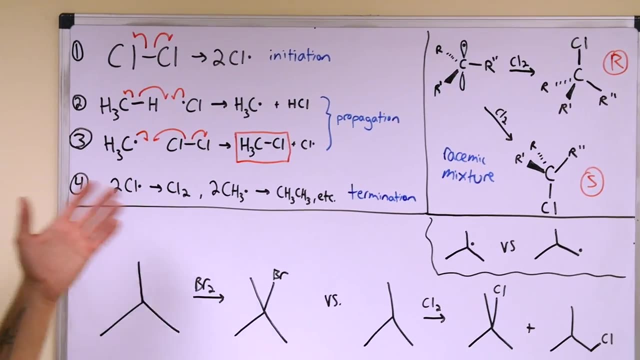 bottom and then the chlorine would now be on the bottom here. well, if we have a, three different groups dictate that we have formed a new stereocenter. so we have to be aware of the possibility of forming a racemic mixture of enantiomers when we are looking at radical mechanisms. so that describes the 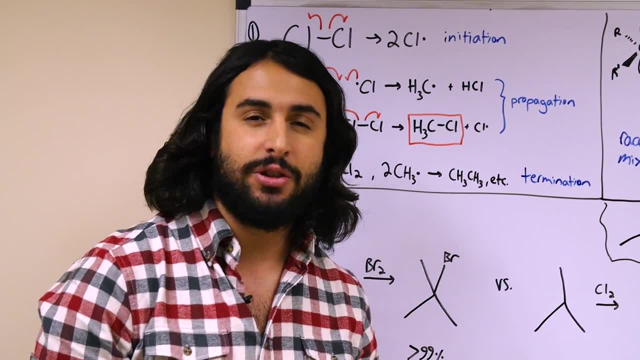 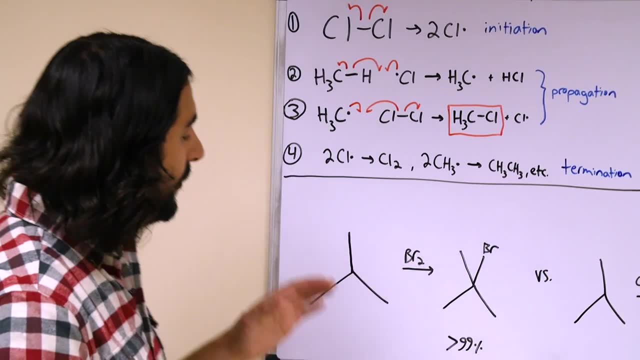 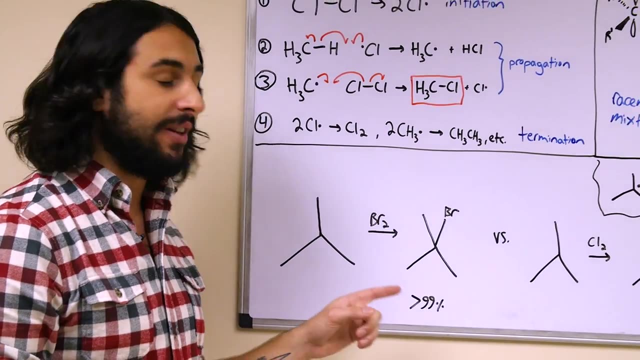 halogenation. now, the other thing that we have to understand about halogenation is that a free radical halogenation can potentially be a very regioselective process, and so what we want to understand here is that bromination up looking to be very, very regioselective because, let's say, we're going to do a bromination. 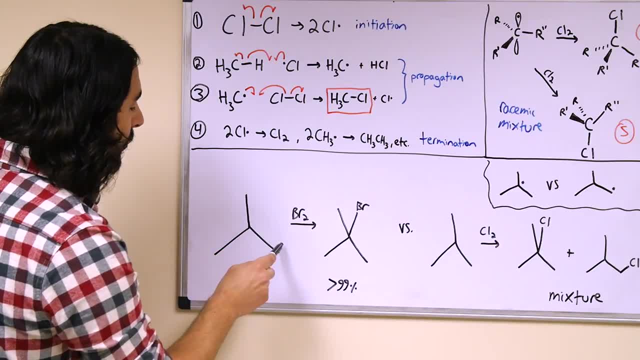 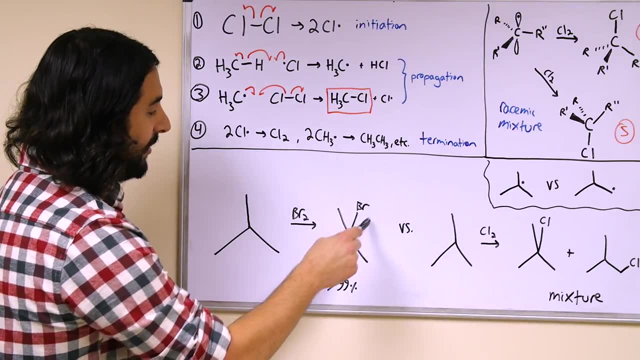 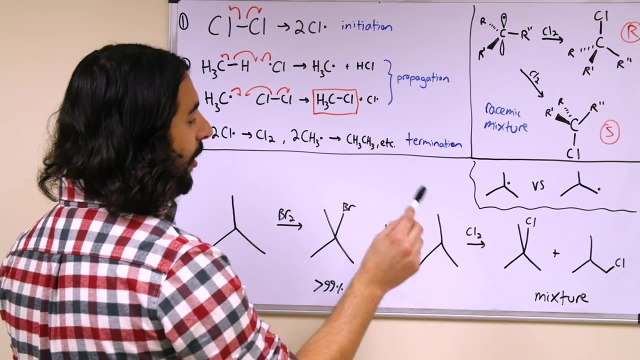 on isobutane. so there are four possible locations for a bromine atom to end up and, as it turns out, we get strictly bromination on this location here, so we get the tertiary system. now chlorination ends up not being so regioselective, we actually get a mixture of the tertiary and the primary. 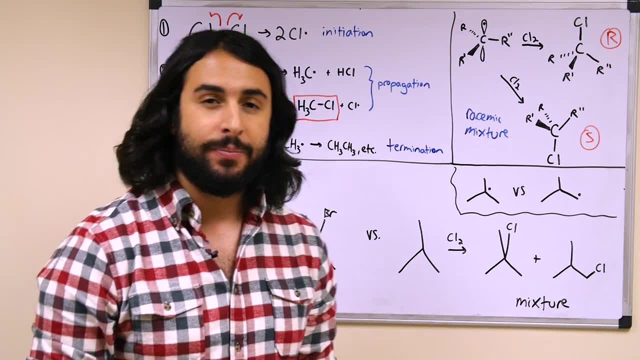 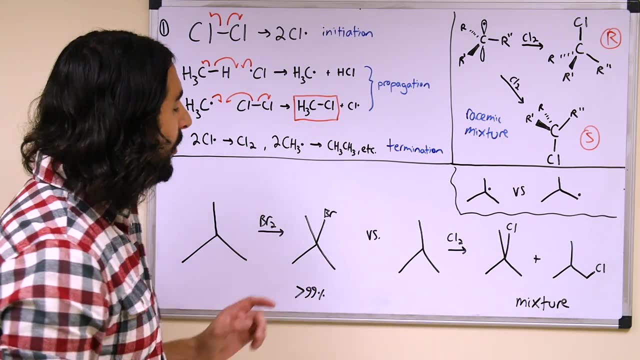 chloroalkane. so we want to try to understand why that might be, because we want to be able to predict product mixtures. so the key here lies in two things. number one: we want to understand the difference in the stability between the bromine radical and the chlorine.